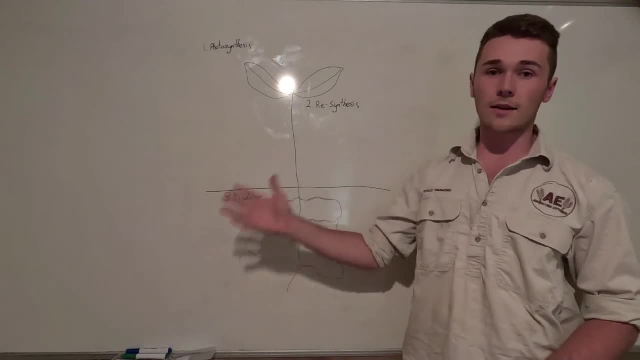 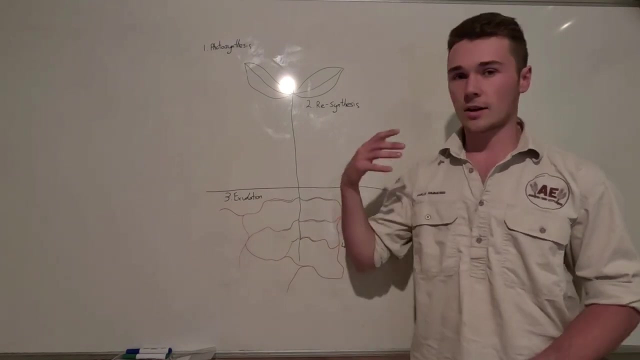 only way to do this is through this process, which was outlined by Dr Christine Jones, And it is what she calls the liquid carbon pathway, And so I'm going to quickly talk about what this is. I've built a whole course around this and more, if you want to go check that. 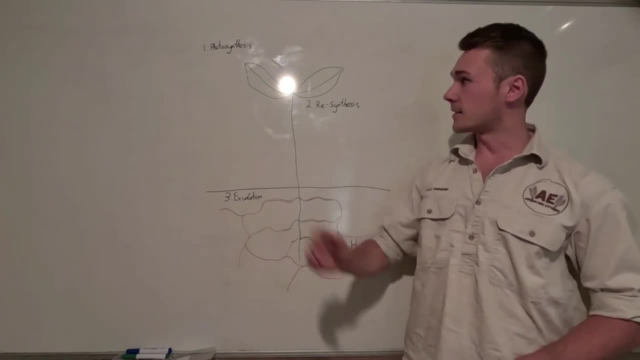 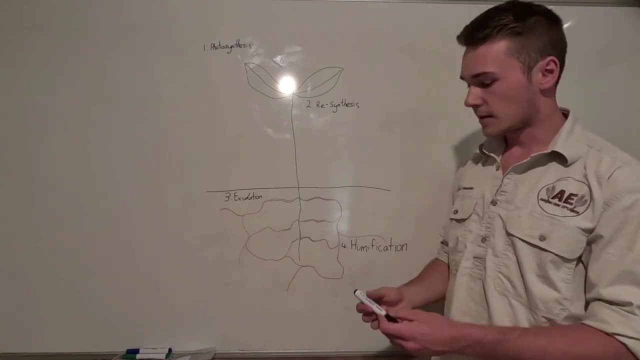 out. It's on the Soil Learning Center. There's a link to that below too, Anyway. so it starts off with photosynthesis. If you don't know what that is, I've made another video on that, So check it out. Essentially, the leaves or the plants are making their own food from carbon in the atmosphere. 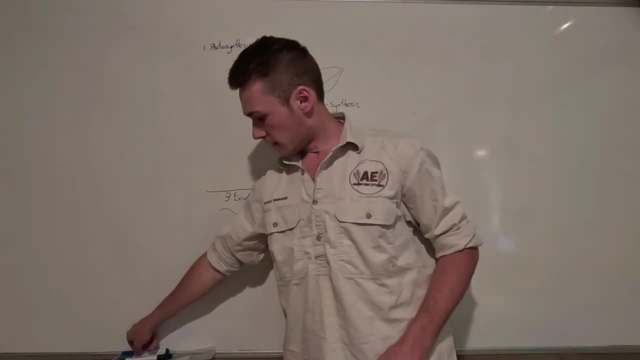 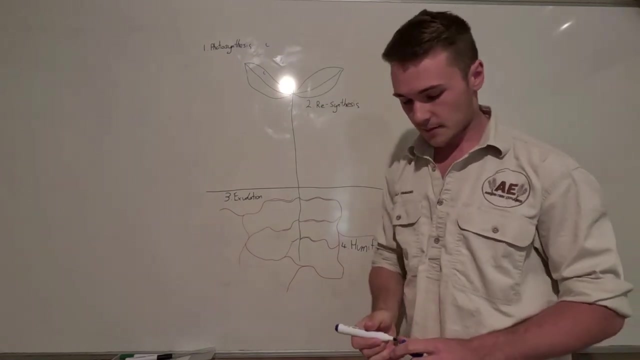 and water, And so, if we think about it, there's carbon in the atmosphere. That's going to be fixed. in our leaves, There's sugar, Then what's happened? So that's our first step: photosynthesis, That's fixing the 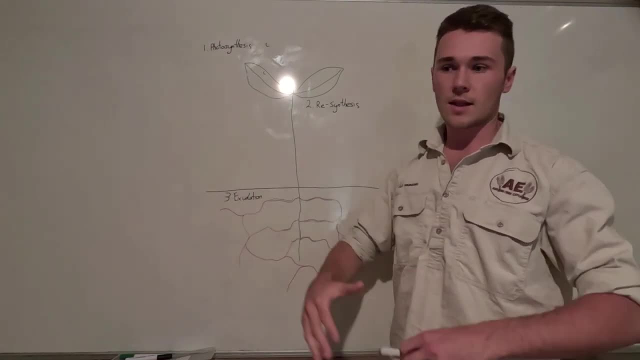 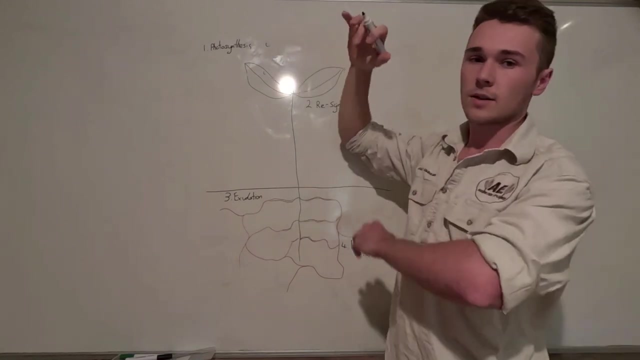 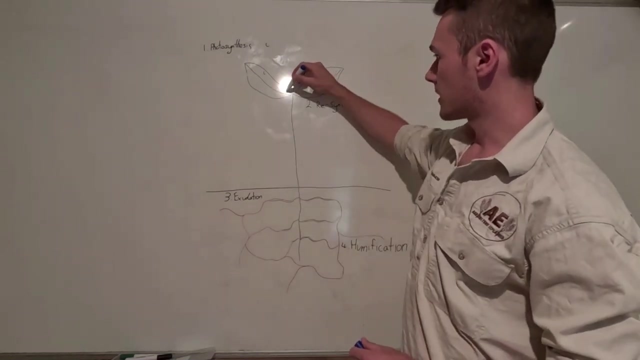 carbon into sugars. Then we have resynthesis, which is that carbon is then remade into other things. So we're taking that glucose or making proteins and fats and lipids and other carbon-based compounds, And so when we're following this carbon, it's resynthesized into different carbon. 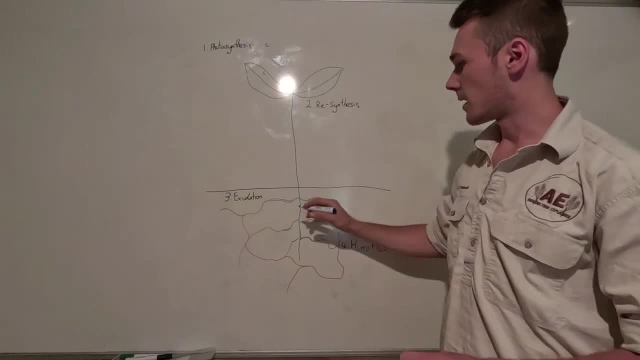 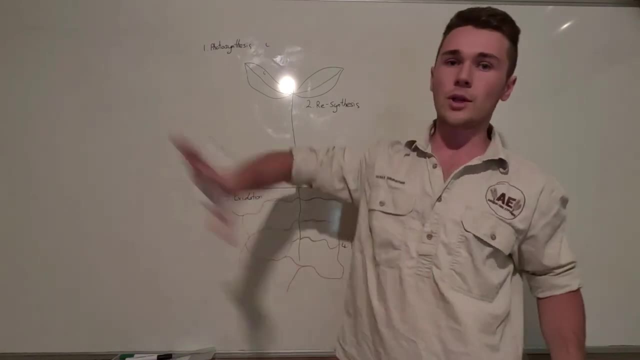 compounds and then pushed down into the roots. Then we're going to our next stage: extradition. This is where the plants throw out. they push out these carbon compounds, And there's a range of what they are, So that carbon is pushed out to the 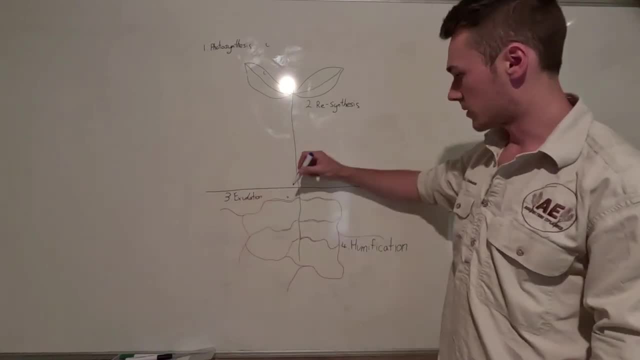 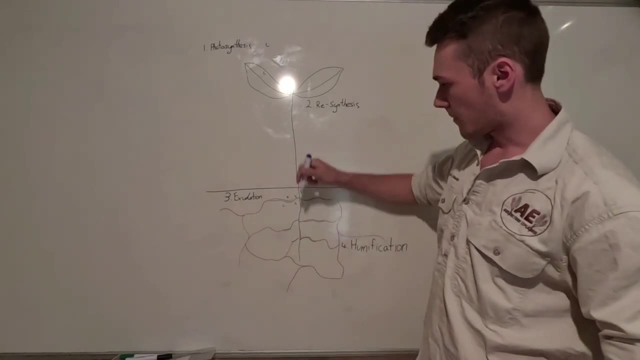 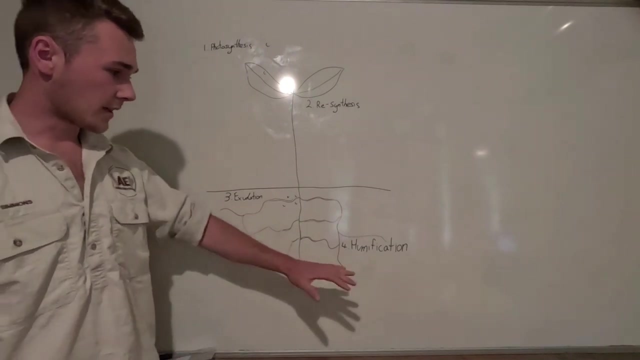 soil for the next stage and for the microorganisms. So now we've got a bunch of carbon surrounding our roots in the rhizosphere, which is that area just right next to the roots. The very last stage is called humification. This is critical. 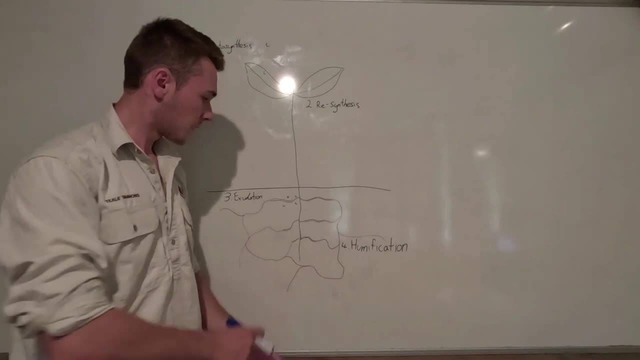 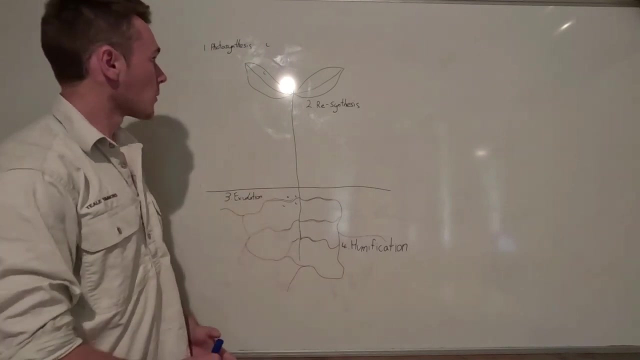 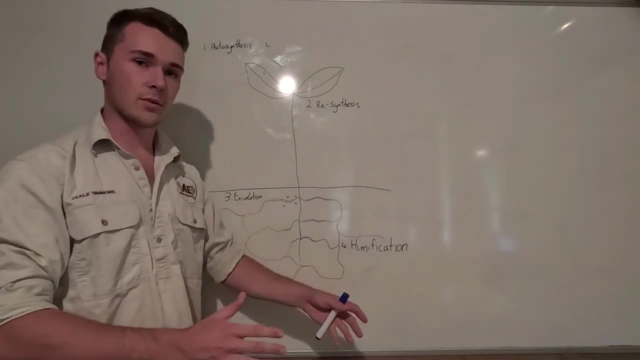 This whole part. This is where mycorrhizal fungi take this carbon sugar, eat it down and then pretty much produce this humic substance, And so we need every single part of this process to produce humic substances which increase a very stable form of soil, organic carbon and arguably the best form of